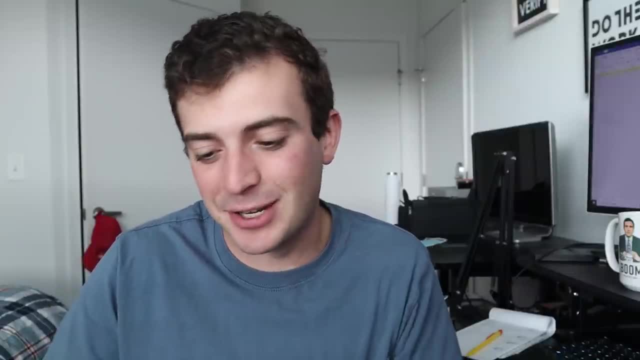 you got to know the periodic table? I think I don't really know. I'm not a chemistry major. Well, the same goes for IT, in my opinion. You get the point. Sure, you can provision a Kali Linux VM. 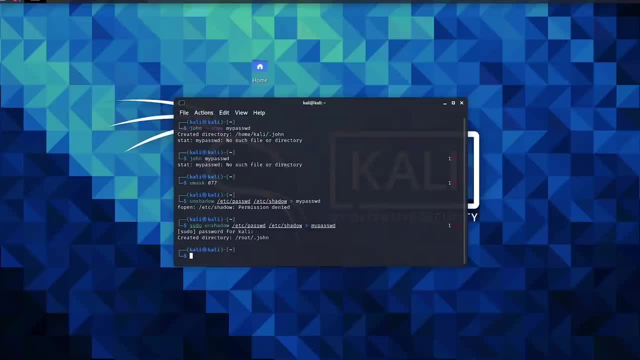 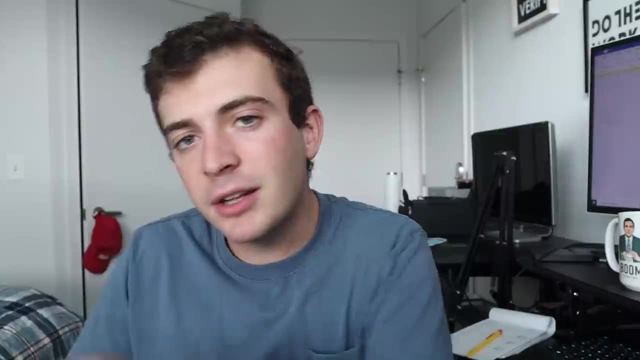 and you can use John Ripper and start cracking those Facebook passwords. Don't actually do that. Or you know you can throw yourself deep into the woods of a project And sometimes that method works. But the question becomes if you have no technological or any IT skills. 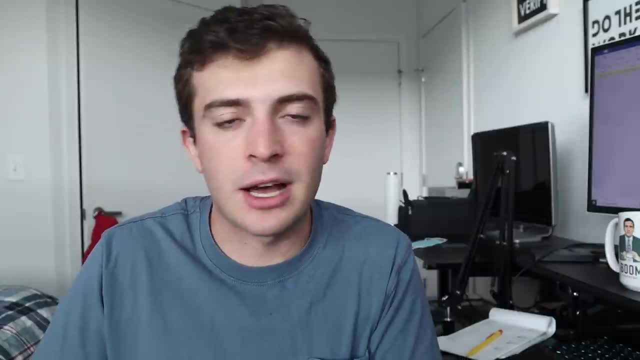 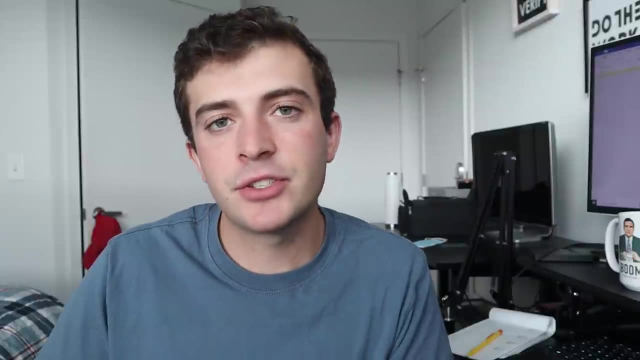 background. how do you know what to secure in the context of cybersecurity if you don't even know how the technology tool principle concept works right? If you can't understand what a layer to switch does from you know, a high-level overview, you're not going to be able to do that. You're not. 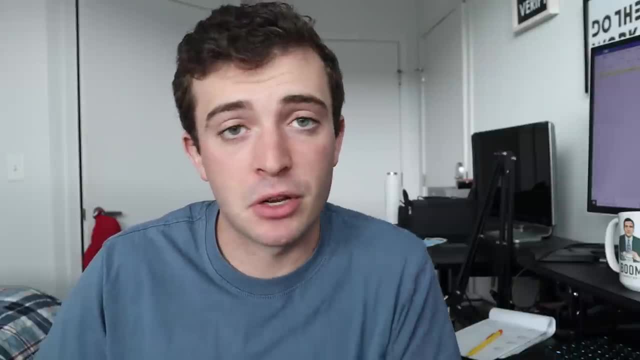 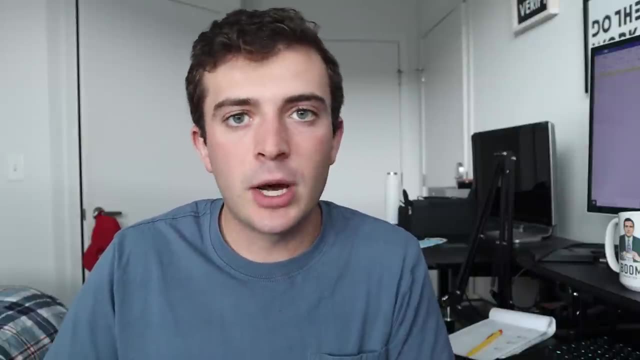 going to be able to do it. How do you know you're going to need to apply port security, you know, in the context of a layer to switch. Well, you won't know, because you don't know how a layer to switch works in the high level, And that's why I suggest the IT fundamentals. It's a great. 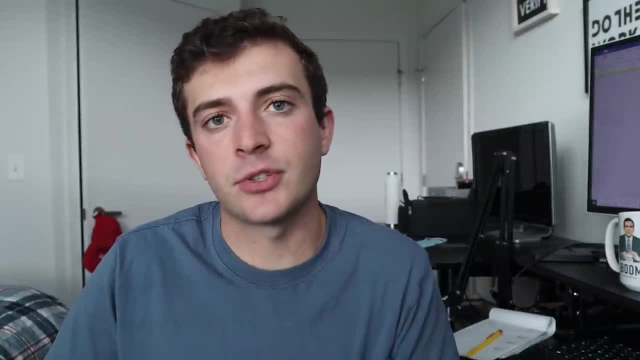 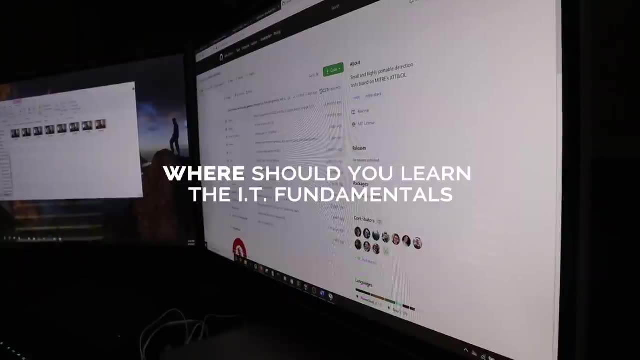 way to get the basics down. You can build those foundational skills and then you can throw yourself into the woods of, you know, Kali Linux if you want to. There are hundreds of resources out there, both free and affordable. All right, one moment of. 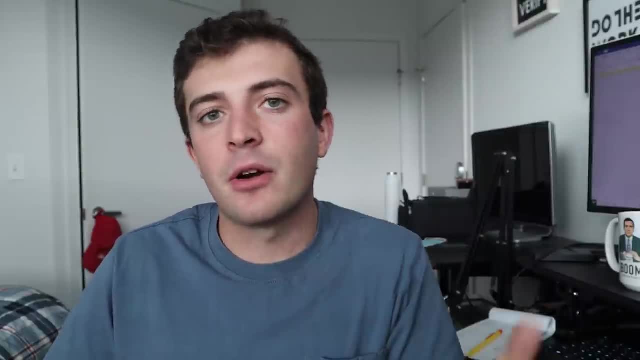 self-promo. You can see what I'm talking about. You can see what I'm talking about. You can see what I'm talking about. You can skip to this timestamp if you don't care about this. But there are three courses I have out there. One is on Udemy. It's a complete introduction to 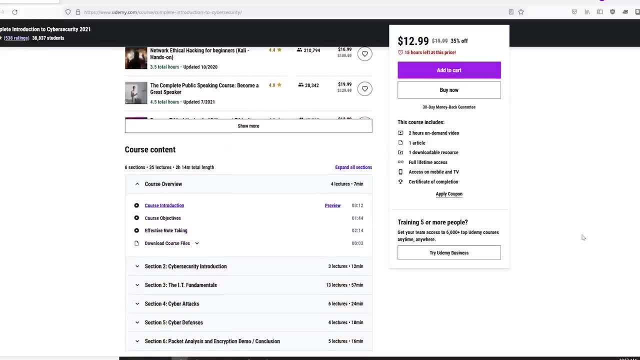 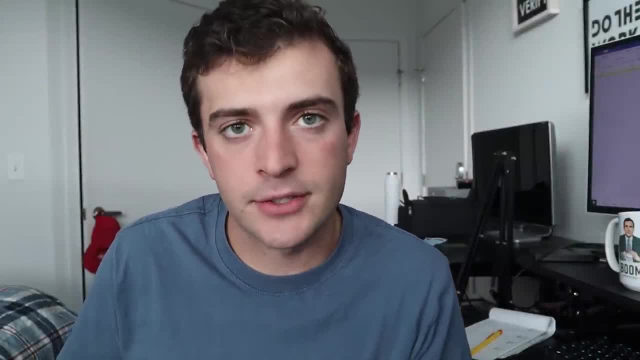 cybersecurity right. So this is going to be a very high-level overview of cybersecurity and IT, And we address some of the very basics, such as hardware and networking devices. So why not just give away the course for free, If you're watching this in the next three days of this upload? 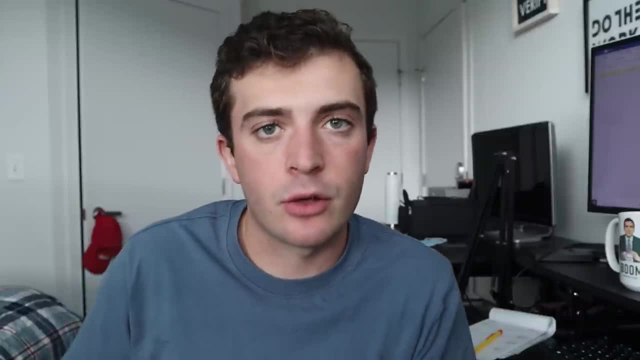 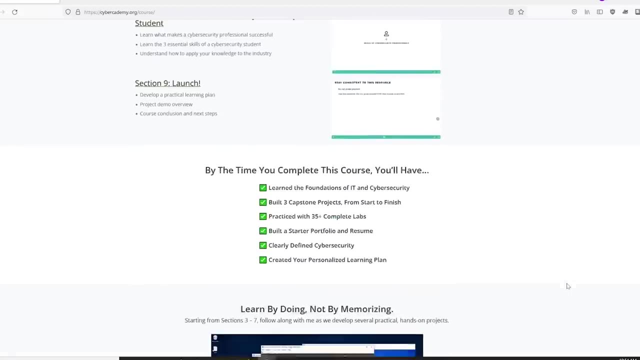 you can go sign up for it for free. But I do also have another course. It's more of a very macho practical hands-on course that I had released last year And I've added some few updates to it. This is a great course to get started. And now enough for the self-promo, All right.